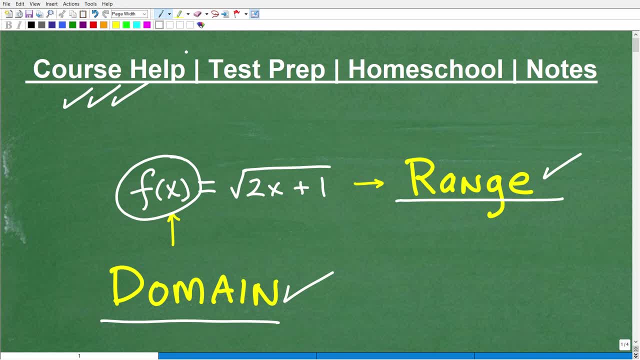 help program. I'm going to leave links to all my stuff in the description of this video. Also, if you happen to be preparing for any sort of test that has a math section, I'm talking about things like the GED, SAT, ACT, GRE, GMAT, ASVAB, maybe a teacher certification exam. 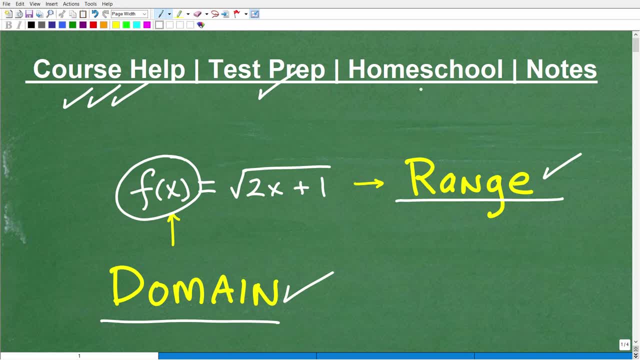 I have a large library of test prep courses you can check out. If you homeschool, definitely check out my middle school and high school math courses. I have a fantastic homeschool program And if you need some math notes, I'm going to leave links to my math notes in the description of this video. 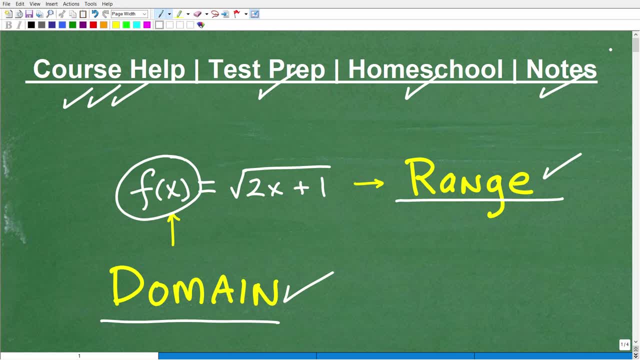 Okay, so let's get going. Domain and range: If you think you know what these terms mean in your own words, put your definition down for what the domain is and the range into the comment section. Because, guess what, You don't have to do that, You don't have to do that. 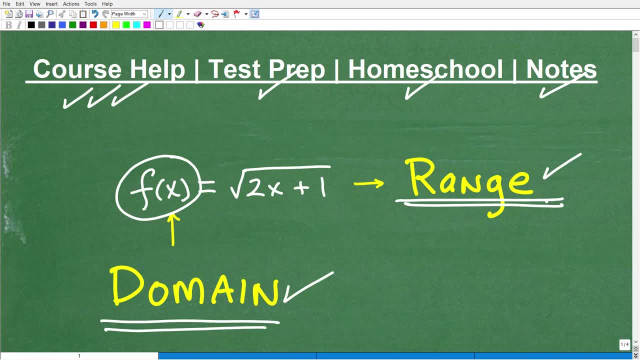 You don't have to have a super technical definition. You know, I think for me, as a math teacher, I would ask you: hey, tell me in your own words what the domain of a function is and the range of a function is. So again, this is a big, big topic, but let's try to make it easy. 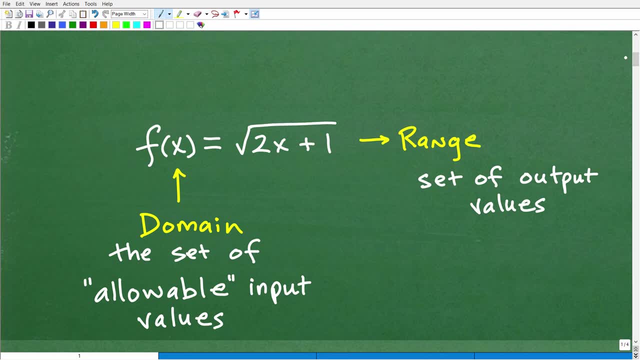 to understand. Okay, so here we go. So here is a function. We are talking about the main topic of functions, okay, in algebra, which is hugely, hugely important. So this, for example, is a function. Okay, we could see here by this little notation, that's f of x. 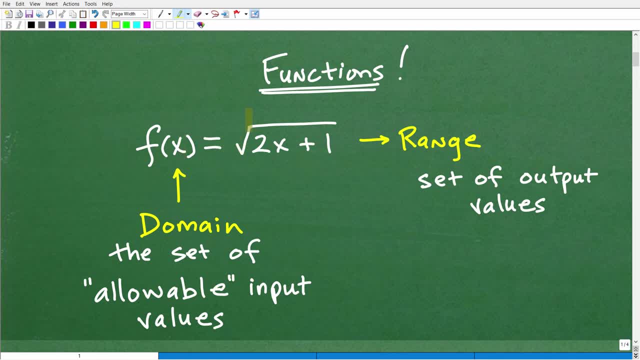 That's a function. So this particular function is: f of x is equal to the square root of 2x plus 1.. Okay so let's talk about this first word: domain. What is the domain? Well, effectively, the domain is the set of all allowable input values. okay, So, in other words, I could put: 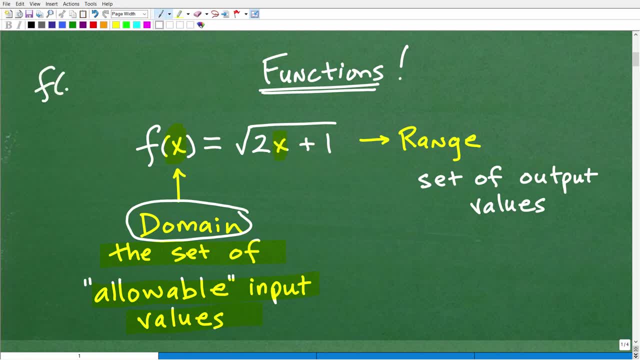 values into this function. In other words, I can go like: all right, what is f of 1?? Well, if I wanted to find f of 1, I could put values into this function. So if I wanted to find f of 1,. 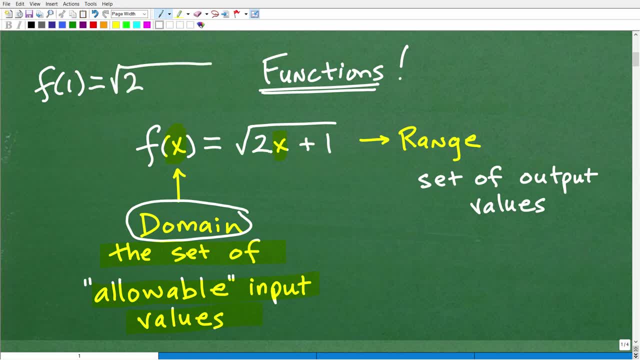 for this particular function, I would just go like: all right, 2,. I'm going to replace this x with a 1.. Okay, so again this x. here you plug in whatever number you want. This is the input value. 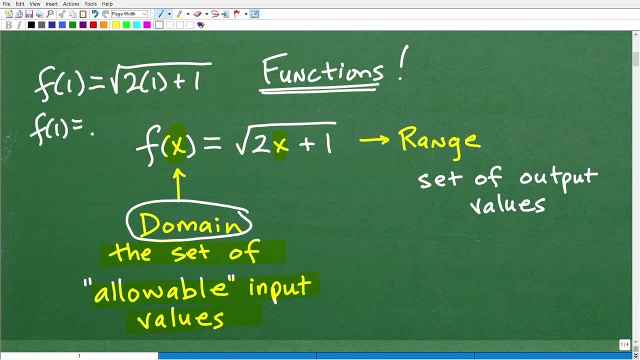 And then I would go ahead and simplify it. So f of 1 would be what The square root of 2 times 1 is 2 plus 1.. So f of 1 would be the square root of 3.. Okay, so 1 was the input value and then 3 is. 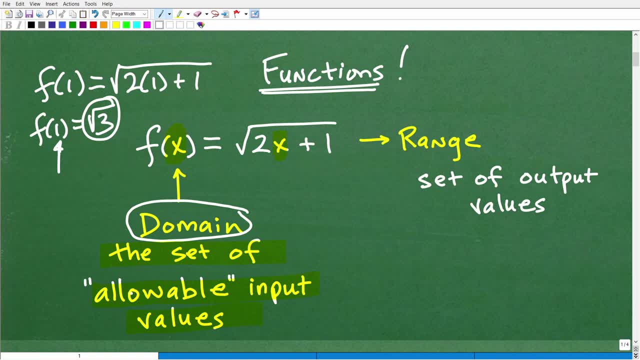 the output value. So the domain, which is the input value, is the output value. So the domain is the set of all allowable input values. I'm going to clarify this here in a second, but effectively that's what the domain is. It's the set of all numbers that we're allowed to plug into. 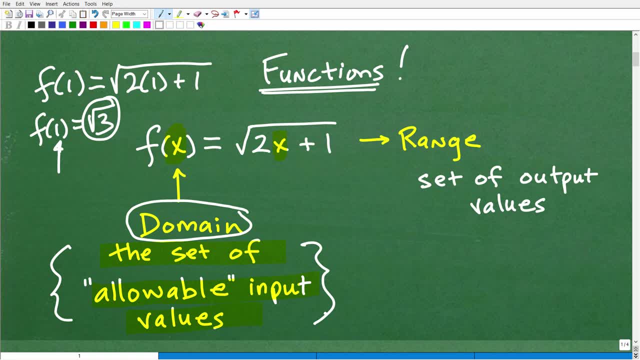 a function. So you might be wondering like: well, can't we plug in any number into a function? Well, this is where I got to give you some additional information, So let's hold on one second to that question. All right, let's talk about what the range is. okay, The range is a. 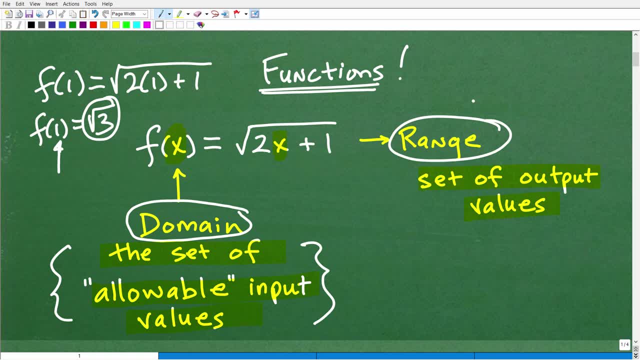 set of all output values, okay, And the range is dependent upon the domain. okay, So the domain is our input values. So, whatever we can put into the function, we're going to get a respective set of output values and that is the range, okay. So this is more or less what the domain and range is. 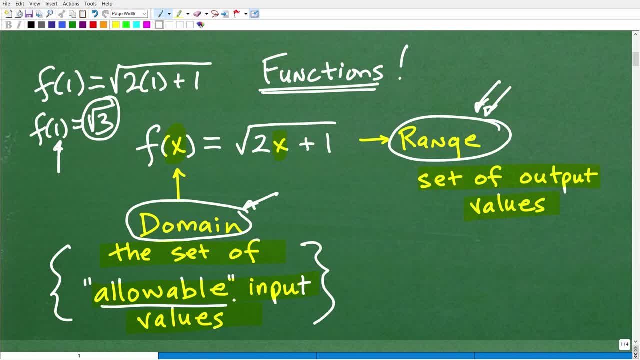 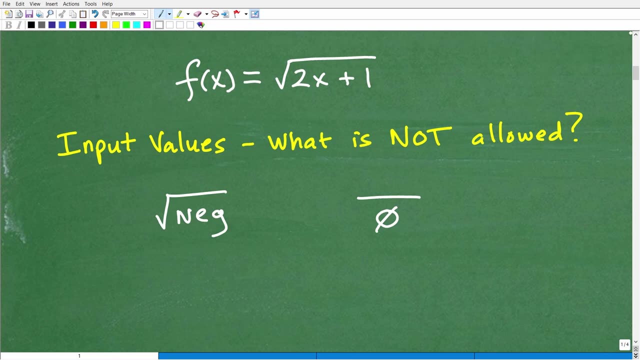 So now let's get back to this question: What is allowable in terms of input values for a function? okay, So that is kind of the main idea here. So let's talk about input values. Well, first of all, let me just clarify when we're looking at the domain and range of functions. 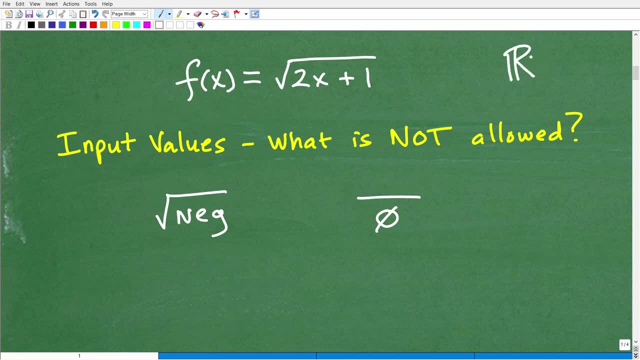 for most of you out there, we're talking about defining the domain and range in terms of the set of the real numbers, ie numbers that are on a number line. So here's zero, here's one, here's two, here's negative one, here's negative two. all the numbers, all the positive and negative. 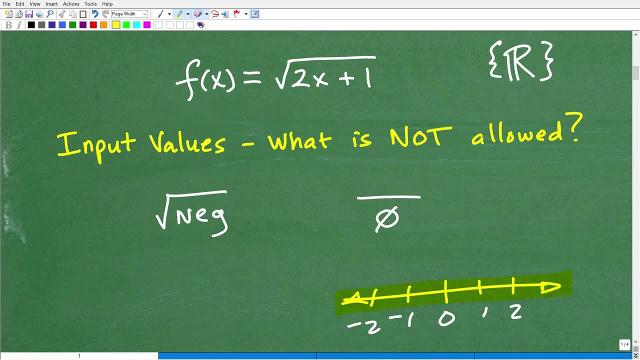 fractions. So we're talking about the set of all the real numbers, ie numbers that are on a number line. So we're going to keep our conversation with respect to what the domain and range is in terms of the set of real numbers, because if we took the complex numbers, which 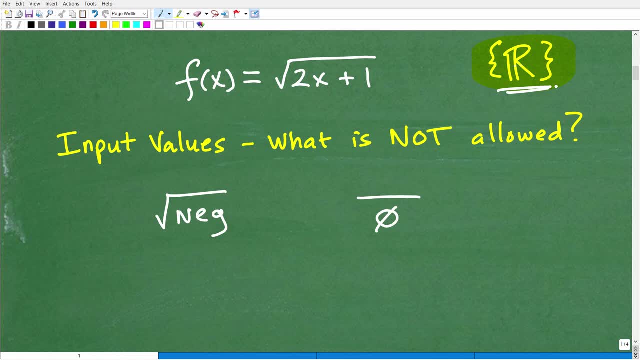 are. we're talking about more advanced math. So, really, again, this video is directed towards those of you that are at the, you know, Algebra 1, Algebra 2 level. okay, So we're talking about the set of real numbers. That's important. Okay, so let's talk about input values. So let's talk. 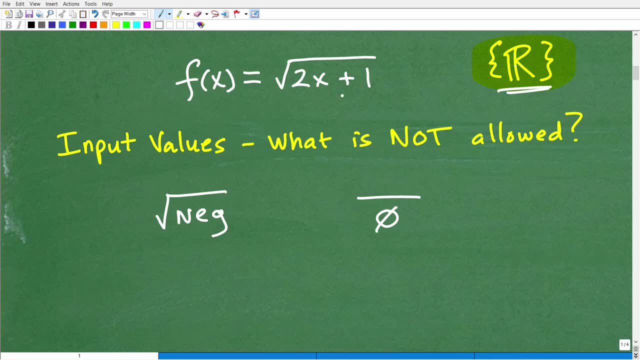 about input values. What is not allowed. Well, effectively, in a function, you should be able to kind of plug in any number, any real number, into a function. For most functions, that's going to be the case. However, when you see a square root, okay in a function like this, well there. 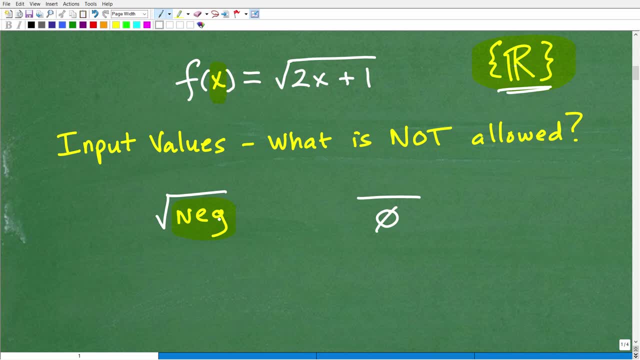 is a condition that you can't have right. You cannot have a negative number underneath a square root. We can't end up with, like negative, the square root of negative 16, because in a set of real numbers, we don't know what the answer is. Now some of you are going to like you're going to. 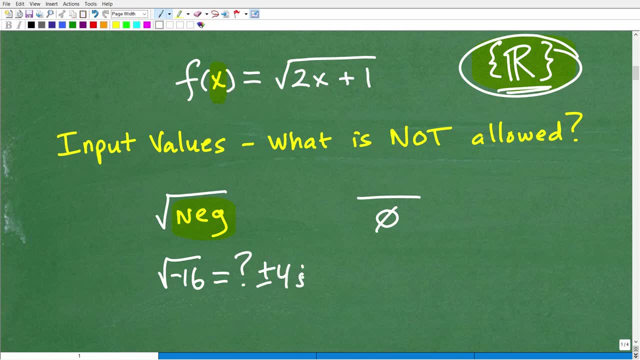 say, oh, that's positive, negative 4i. Well, this is an imaginary number. This is the set of complex numbers. We're not talking about that again. So again, you know. obviously some of you know that the square root of negative 16 is plus or minus 4i. But here, in the real numbers, we can't do. 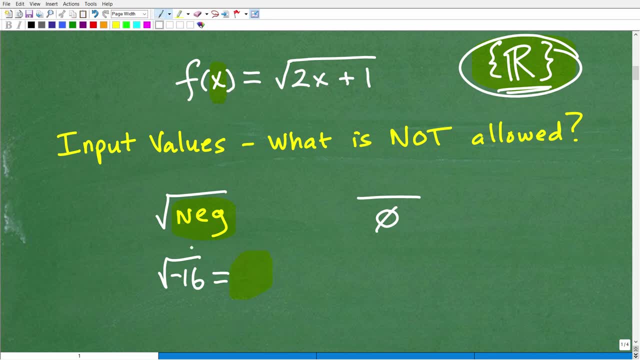 this problem right. So we cannot have a situation where we end up with a negative value underneath the square root. So this is not allowed. So any input value that we'd like, hey, let's plug this number into this function- and we end up with this situation: that number is not allowed. 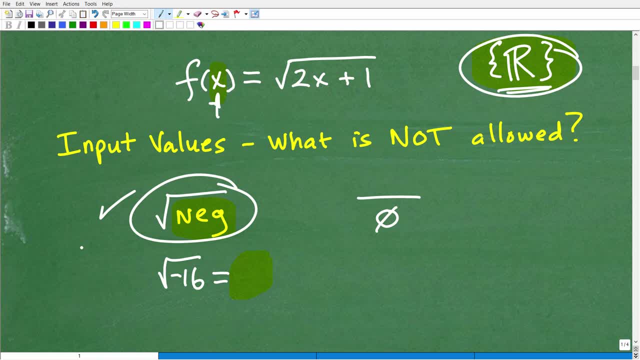 So we've got to like take that out, okay. The other situation is where if we have a fraction- let's show you a problem like this- Let's say I have 5 over x minus 1.. So any function that has a fraction, you cannot have 0 as a denominator. So what value in this particular function would 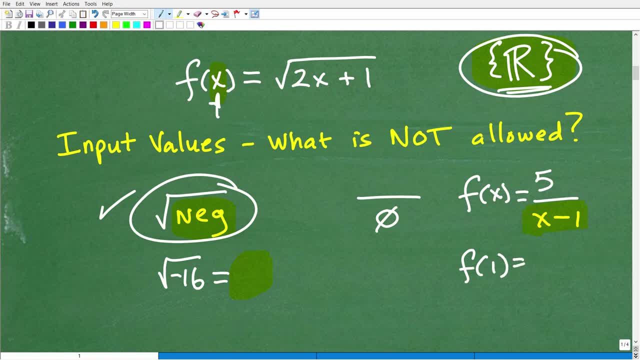 cause that. Well, if I was trying to find f of 1,, I would have to have f of 1, and I would have to plug a 1 for this function. I would plug a 1 right here, right, And I would end up with 5 over. 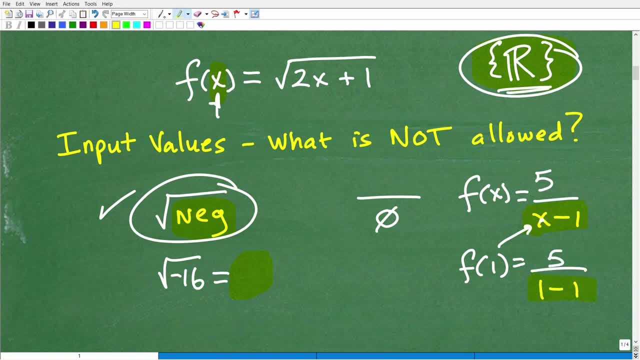 1 minus 1.. This would blow this function up. This would not be good because I would end up with 5 over 0, okay, This is not allowed. You cannot divide by 0 in mathematics, okay. So what input? 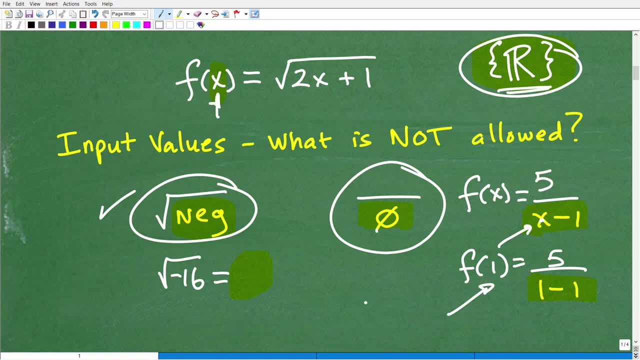 value caused this to be a problem. Well, 1 did So. 1 cannot be a part of the domain. okay, 1 could be a part of the domain for this particular function. Any number is fine except for 1,. 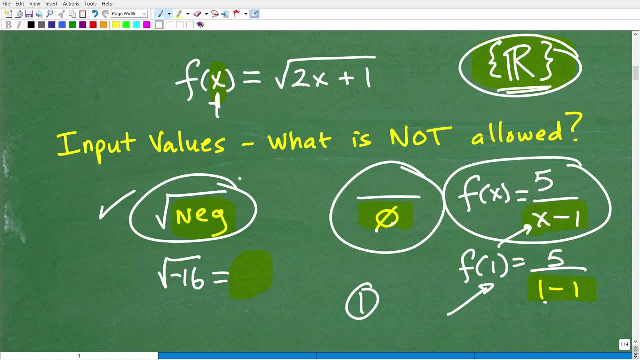 because 1 would cause that to blow up and we have no square roots, so we don't have to worry about a negative value underneath the square root. okay, So these are the big picture ideas when we're talking about what is not allowed in terms of the real numbers in the domain. 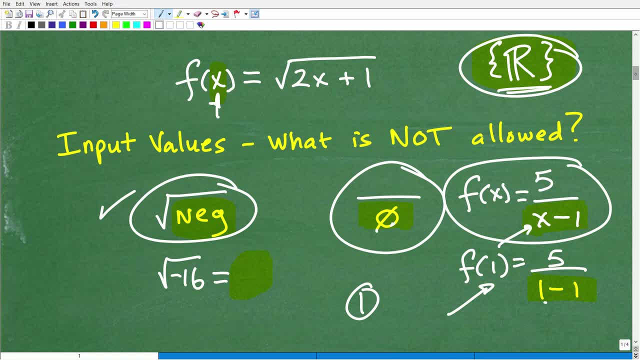 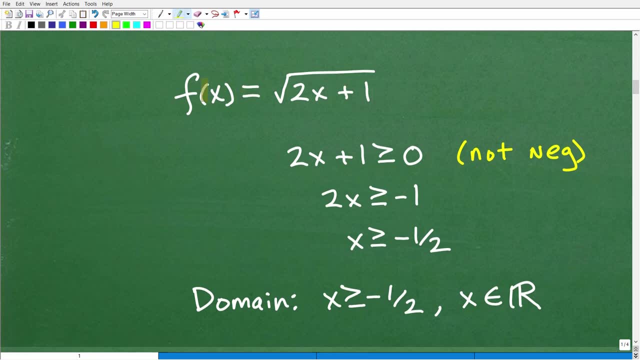 okay, So let's go ahead and work on this a step further. I know I'm covering a lot of ground, but this is all super important information. So let's suppose I said, hey, find the domain of this function okay, We're talking about the same function. 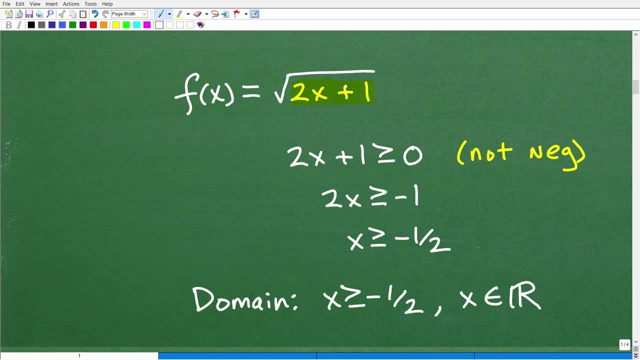 So you're saying, all right, that YouTube math man told me that I can't have a negative value underneath the square root. okay, I can't have that. So, if I can't have that, but what can I have? Well, I can have a positive or 0, okay, Because the square root of 0 is 0. So I'm going. 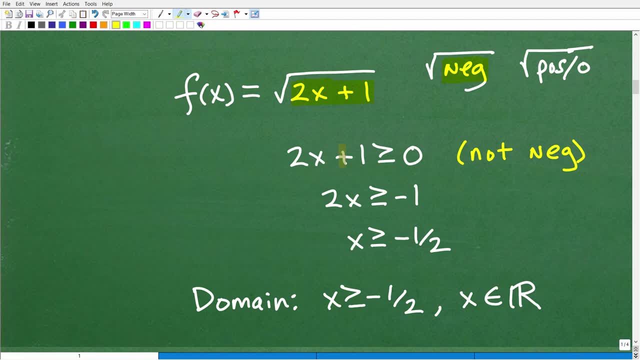 to say: all right, so 2x plus 1.. Uh what? when is it greater than or equal to 0,? okay, So 2x plus 1, that whole expression there, that value. when is it greater than 0?? That means it's positive, right, It's greater than 0, or? 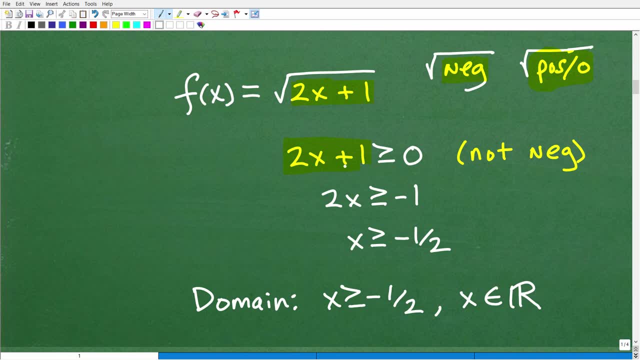 equal to 0.. So we want to figure that out. okay, What x values? um, you know, have 2x plus 1 greater than or equal to 0, ie, it's not negative, because that's what we want. So we're just going. 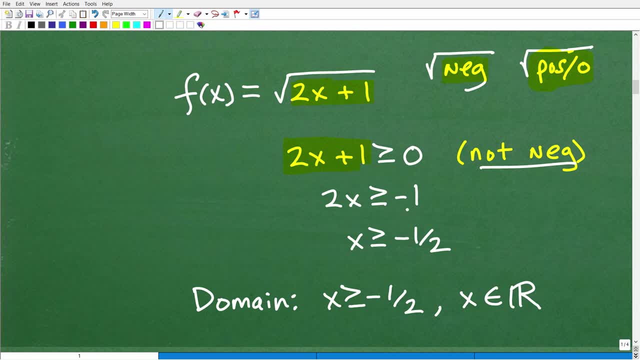 to solve this basic inequality just like an equation, I'm going to scoot that 1 over to the square root. okay, 2x is greater than or equal to negative 1, or x is greater than or equal to negative 1 half. Now, if you don't know what I did here, right? uh, in this little basic uh. 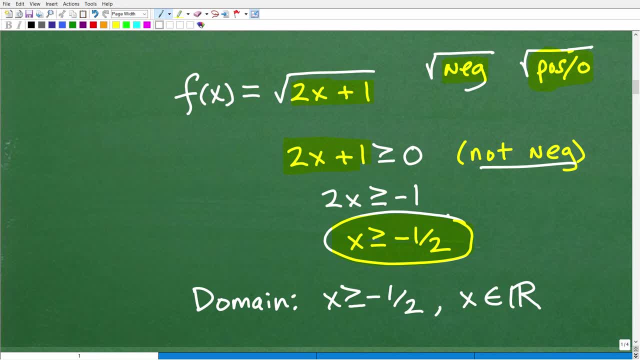 inequality, then you know, mark that down in your terms of your list of things you need to review, because you need to understand this in order to, uh, figure out what the function or the domain is of functions. okay, You got to understand basic inequalities, etc. Okay, so all. 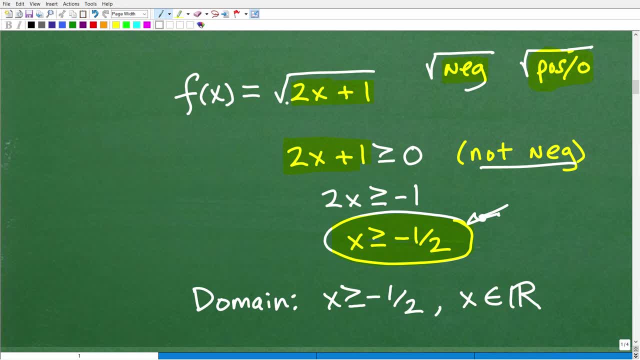 x is greater than or equal to negative 1 half. We'll cause this thing right here to be not negative 0 or not negative, and that's what we want. So we can define the domain to this function as all x is greater than or equal to negative 1. 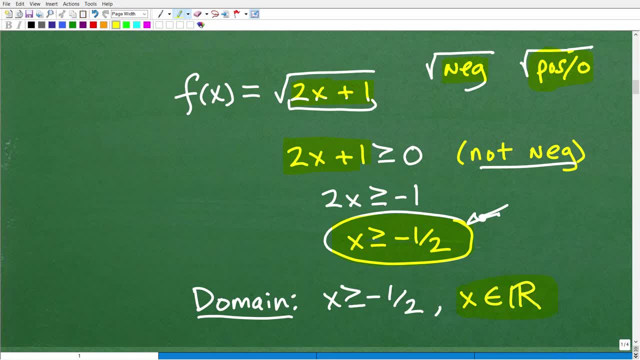 half, where x is um an element of the real number. That's a little technical thing, just saying x is a part of the real number, uh system. okay, So there's other ways we can define the domain. but uh, if you kind of gave me this answer, I would say you are awesome. Matter of fact. 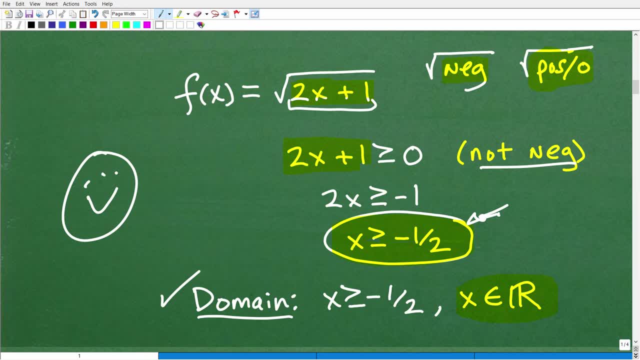 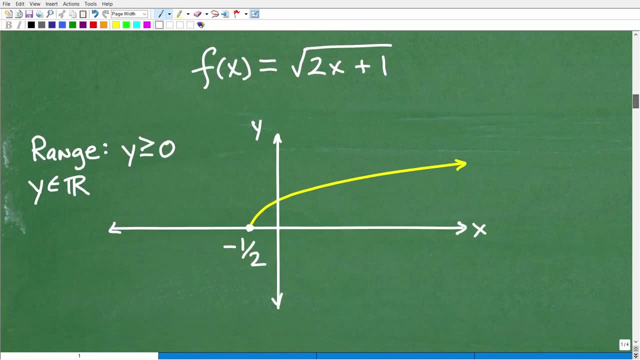 I'm so happy face for being such a great uh math student. okay, So let's move on and talk about the range now, okay, And we'll kind of wrap this up. The range is a little bit more difficult to uh find. okay, Uh, and the range. the easiest way to find the range oftentimes is by looking at. 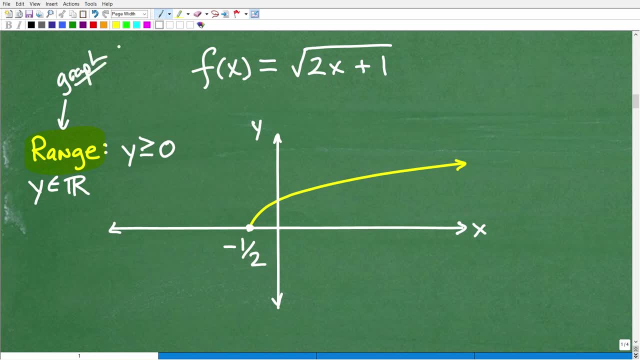 a graph. okay, So the domain is easier to find than the range typically? uh, because the range? again, the easiest way to do this is to look at a graph. So let's take a look at this function again, same function, and uh, of course, 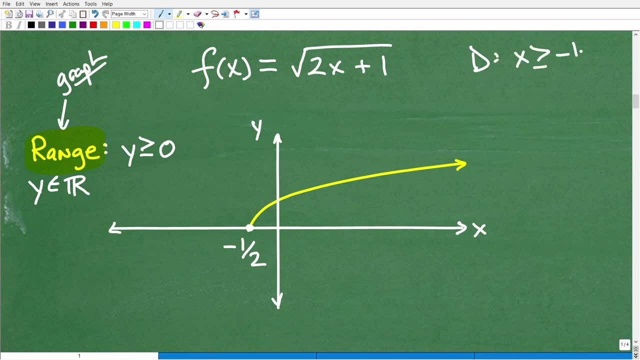 we know, the domain is all x is greater than or equal to negative 1 half. We are talking about the real number system. So here is the graph. This happens to be the graph of this function. Now notice where it starts. It starts here, at negative 1 half, and it kind of goes like this: 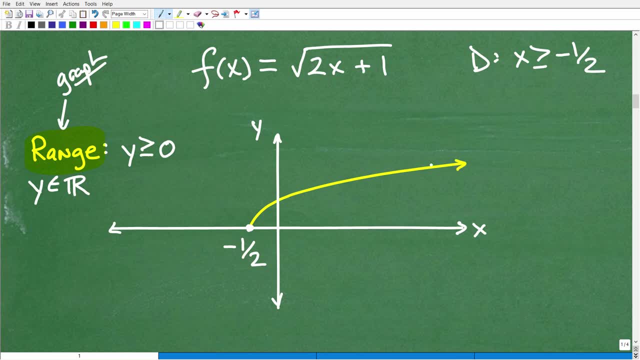 arcs this way. Uh, this is what a square root function looks like, if you didn't know. So this happens to be the graph of this function. Now let's look at the x-axis. okay, You can see. it starts from negative 1 half and it goes. 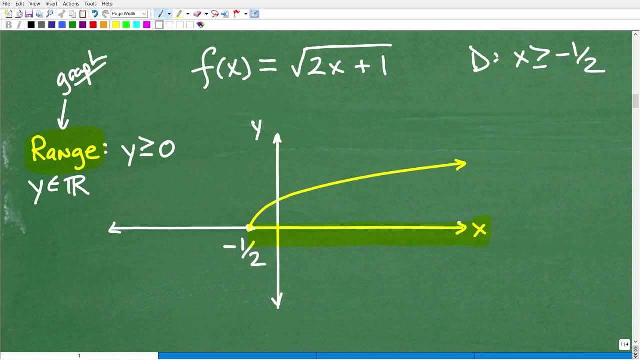 all the way to the right. So all numbers greater than or equal to negative 1 half are by x values. okay, This is, uh, the domain, okay, But the associated output, which is the graph itself, is on the y-axis. So what y's are being covered here? Well, it starts from zero. 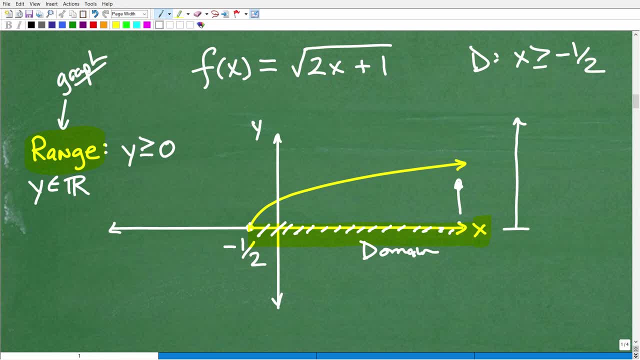 and this graph is going up and up and up. In other words, these y's right here are on this graph. In other words, that point there is: uh, a y, um, a y. coordinate all these points here. And, of course, this thing: 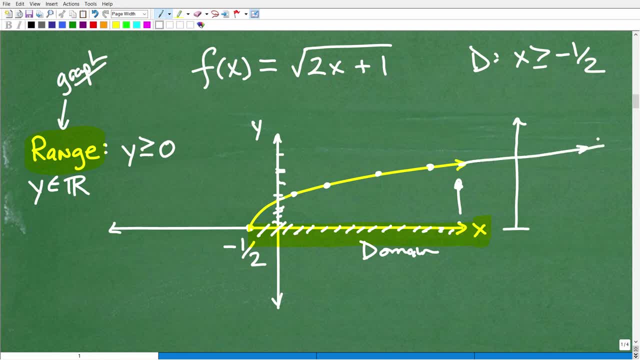 goes up infinitely high. okay, It will continue to go on and on and on, Although, uh, you know it's a little, it's growing kind of slowly, it's still going to go infinitely high. So all the entire uh, positive y-axis, these y values here is: 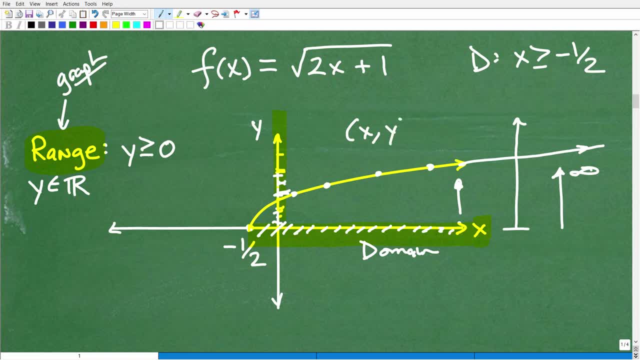 these are the ranges. okay, So an x and y point on this graph. the x values, like this, represent um. these are the input values. This is part of the domain, And then the y values are the associated output values. I'm going to talk about this- this here a little bit more in a second. 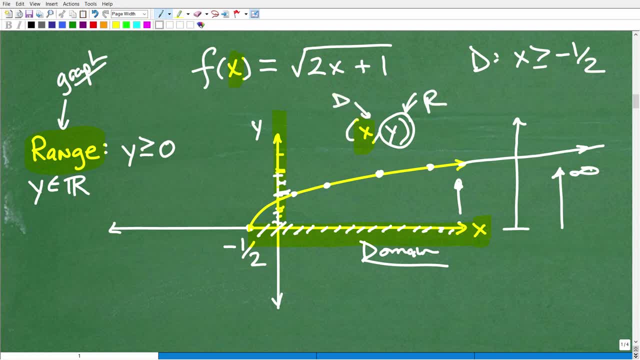 This is the range. okay, The x value is the domain. So, looking at this graph: okay, this graph is going to cover this. when we're looking at, when we're talking about the range, we want to look at this as a graph span with respect to the y-axis. okay, So this is going to be starting from. uh. 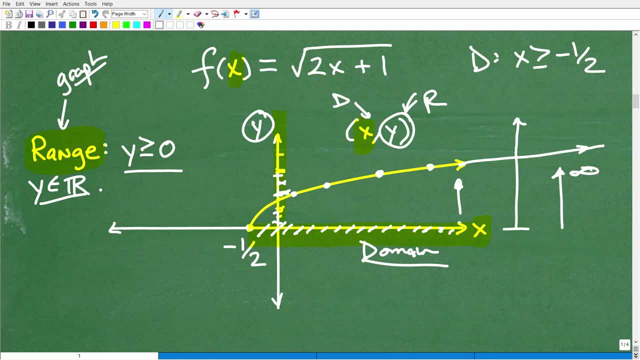 zero. All y is greater than or equal to zero, where again y is a real number. okay, That is the range. This is the set of all output values based upon all these input values. okay, So again, this is a big topic and I'm kind of covering a lot of stuff. uh, quickly, If you, 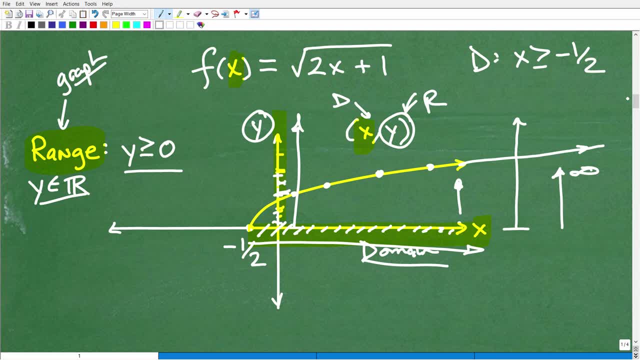 really, really need to master this stuff. I would definitely check out any one of my courses from Algebra 1, Algebra 2, College of Algebra- If you're much more familiar with Algebra 1, Algebra 2, maybe even my pre-calculus course, because I get even more heavy duty into functions. But let's go. 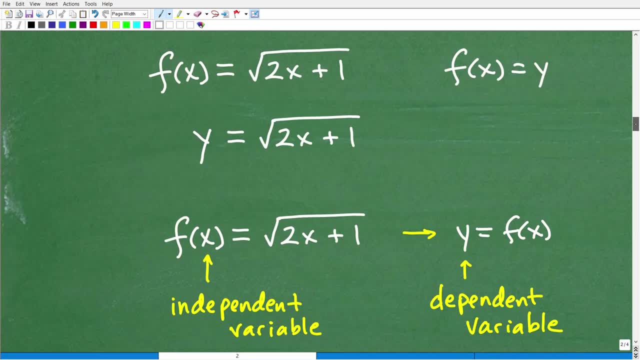 ahead and talk about this here, uh, in a second, and give you one more term, so, uh, that you need to know terms, actually that you need to know. So here's our function. again One thing you need to know: that this f of x, okay, is the same thing as y. f of x is equal to y. So when we plug in an 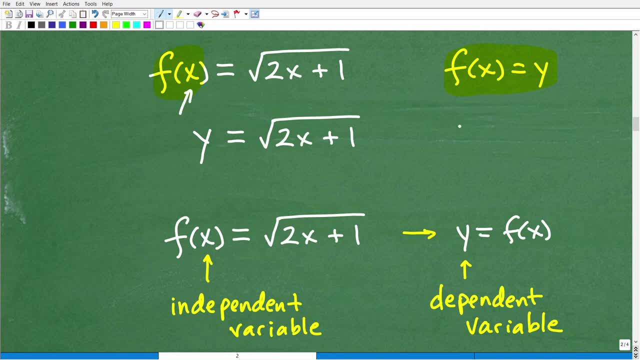 x value this: uh. f of x is the same thing as y And uh. so it's like okay when I have an x and a y whenever I plug in 1,. okay, right there, if I plug in a 1,. 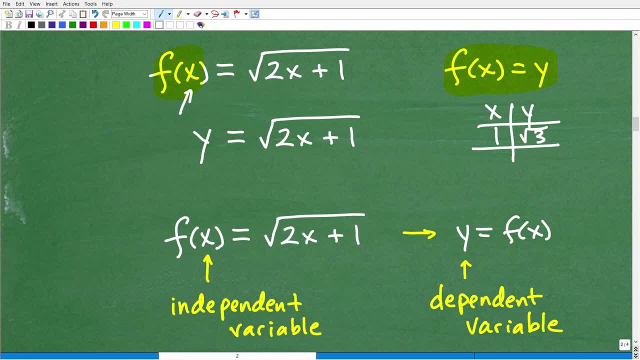 I'm going to get a square root of 3.. y is equal to square root of 3.. We already covered that in the beginning of the video, But this is an xy point. that's on, uh, this graph 1, square root of 3,. 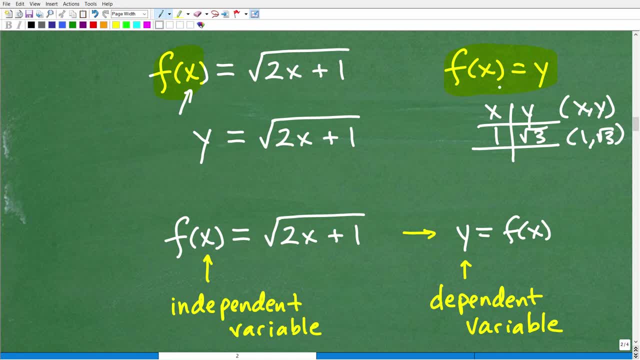 okay, So just so you know. uh, this notation, you understand it. uh, fully, all right, So y is the same thing as f of x. So we're dealing with x and y, So the x just to kind of reinforce. 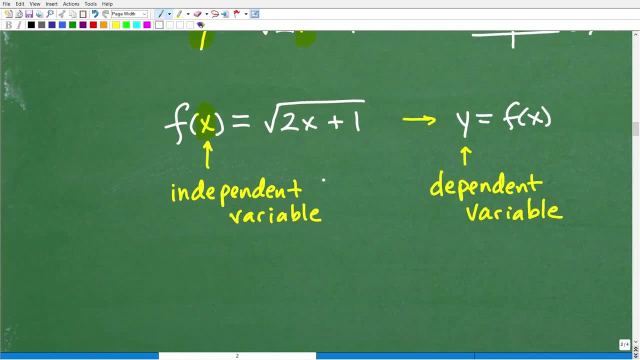 talking about with the graph. this is something we call the independent variable. okay, So we're talking about xy points here. The x's are the independent variables. These are all part of the domain. They're the input values, allowable input values into a function, And once we evaluate, 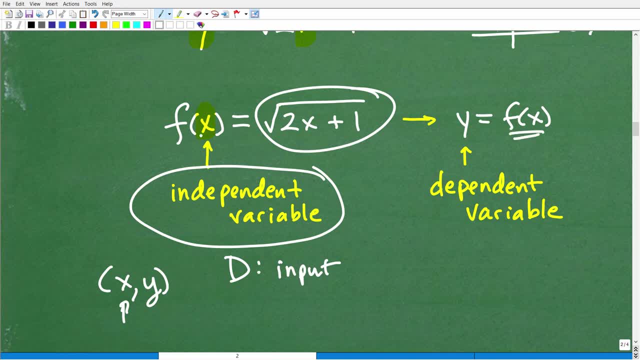 this function. okay, we're going to get an output value f of x, We're going to figure that out, but that's the same thing as y, okay, So, uh, y is the independent uh value And the set of all those values is called a course, called the range. So 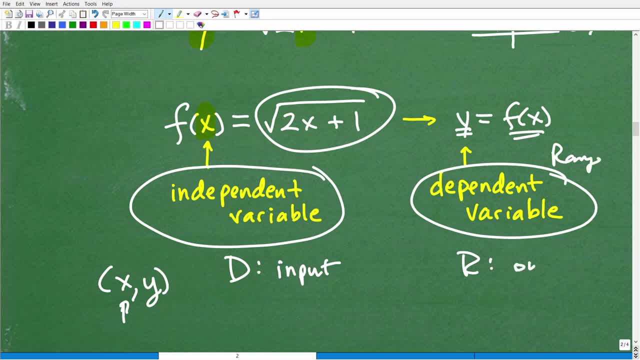 this is the range, okay, And this is the output values. all right. Output values, uh, dependent upon the input values, And there's a lot of different ways we can study this. We can look at mapping diagrams, et cetera, But I'm going to go ahead and call this video a wrap, right here. 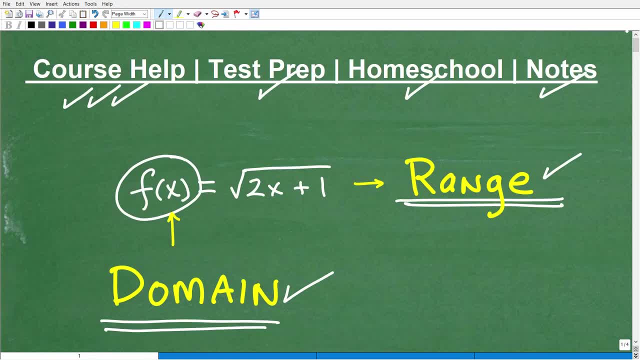 um, because I did cover quite a bit of stuff. But if you understand everything I've talked about here, you've got a pretty good grounding on what the domain and range of a function is. And if you're like, awesome, I understand this, Well then, let me give you a nice little happy. 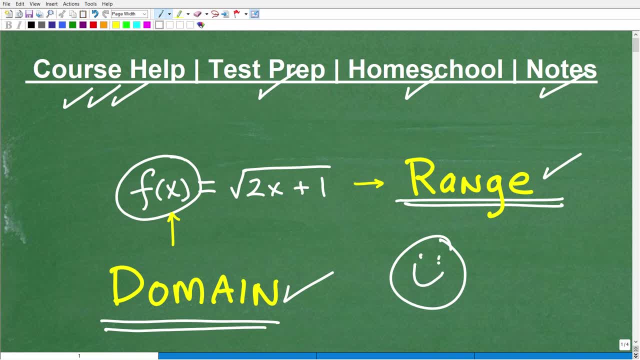 face for being such an excellent math student and paying attention. And, by the way, if this video did help you out, go ahead and consider helping me out by smashing that like button and maybe even subscribe it to my YouTube channel. I've been on YouTube for 10 plus years. I have over a thousand. 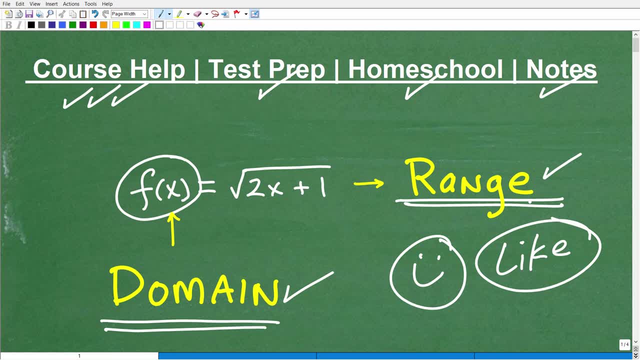 plus math videos on my channel, from basic math to advanced math, like calculus and everything in between. So if you'd like my teaching style, please take advantage of my comments. I'll be happy to answer any questions you may have And I'll see you in the next video. 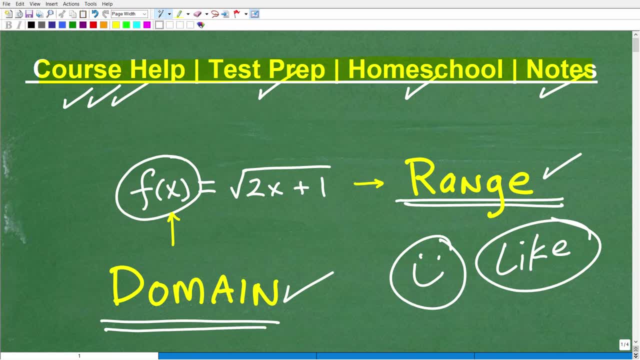 Okay, So, with that being said, I definitely wish you all the best in your mathematics adventures. Thank you for your time and have a great day.